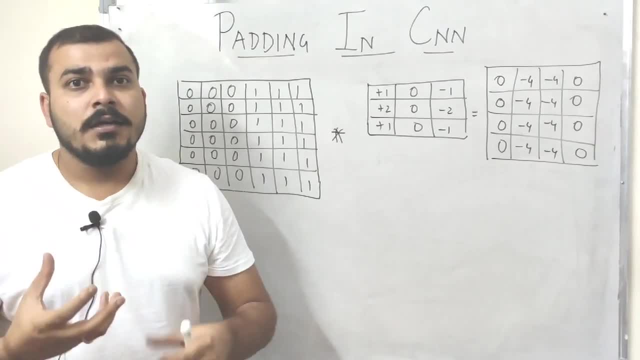 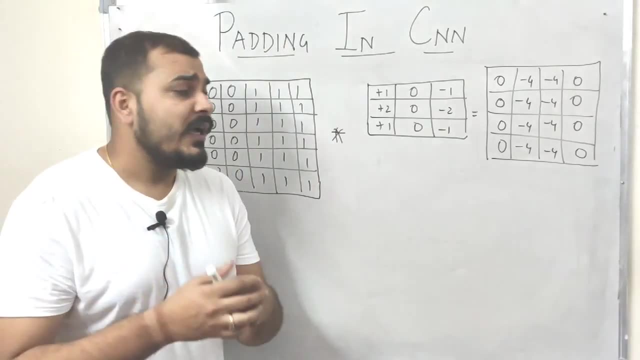 I have already shown you how does convolution operation takes place. So let me just revise little bit of convolution, how the convolution operation takes place, and then we'll continue. with respect to the padding, So I took an example that I had, an image which was basically 6 x 6. 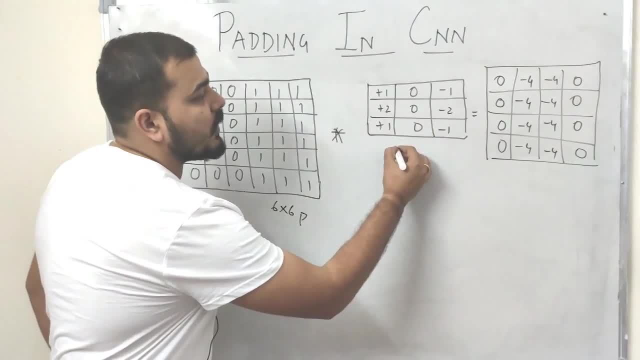 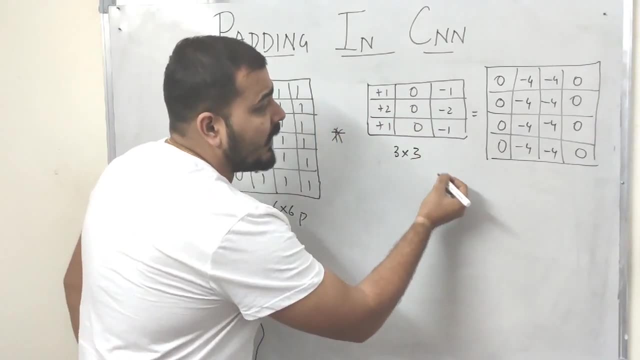 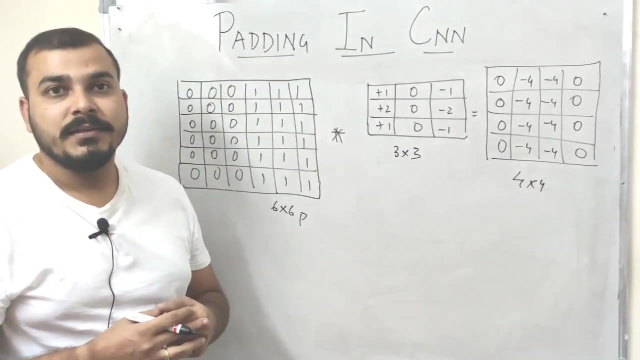 pixels- okay, 6 x 6 pixels- and then I was applying a vertical filter which is basically 3 x 3 of size and over here- and this is vertical edge filter, sorry- and the output that I was basically getting was a 4 x 4 pixels output. Now you need to notice one thing over here, guys: 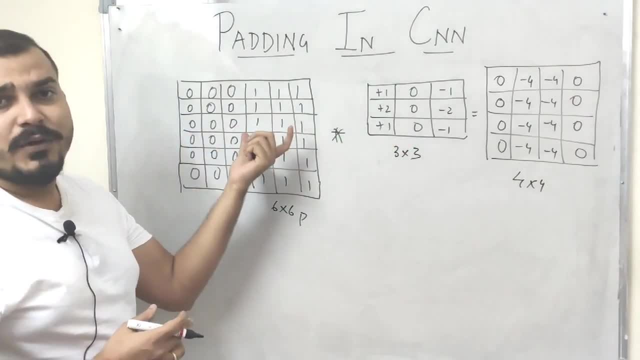 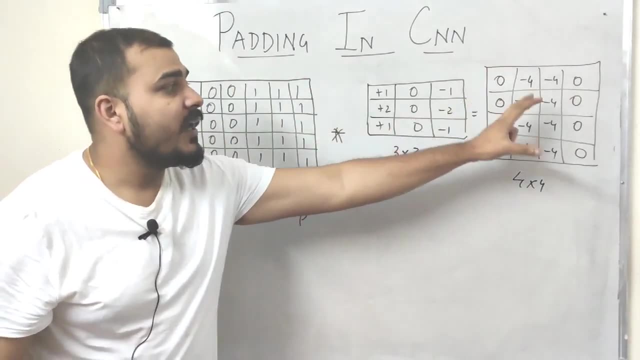 this kind of convolving operation is basically used from strides- right, We were basically jumping from one place to the other place. we are doing the multiplication operation, plus we are doing the summation of all the values and finally we were getting the output. 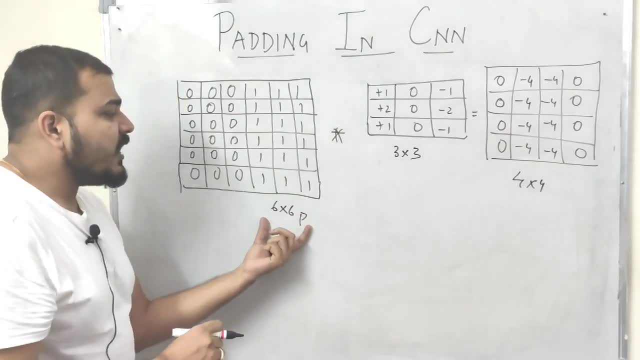 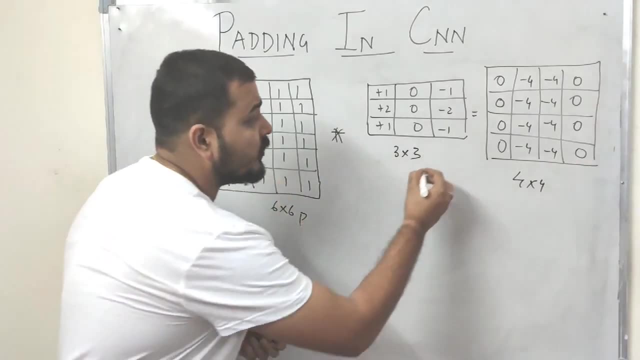 Now one thing you have to note over here: initially I gave a 6 x 6 pixels, and when I applied a filter of 3 x 3, this filter may change. okay, we may also have a 5 x 5 filter. 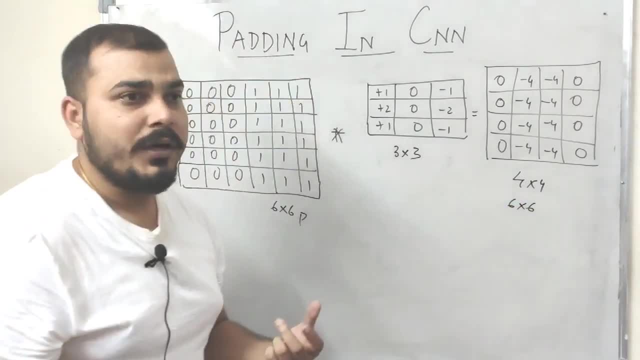 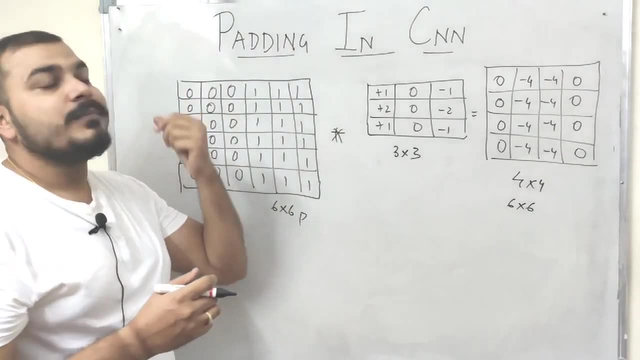 want that, i will be able to get 6 cross 6 pixels output only from my 6 cross 6 pixel of images at that time. if you want to get this kind of output, we basically have to apply something called as padding. now, if you remember my formula of calculating this output dimension with respect. 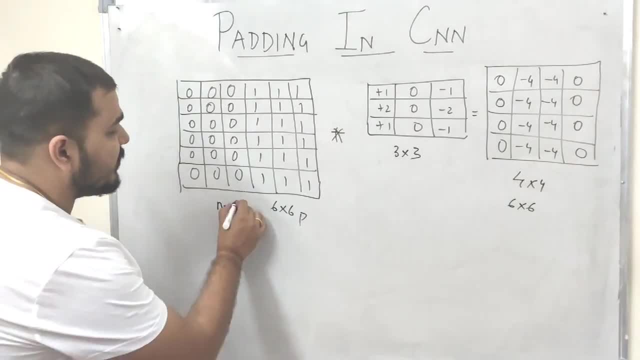 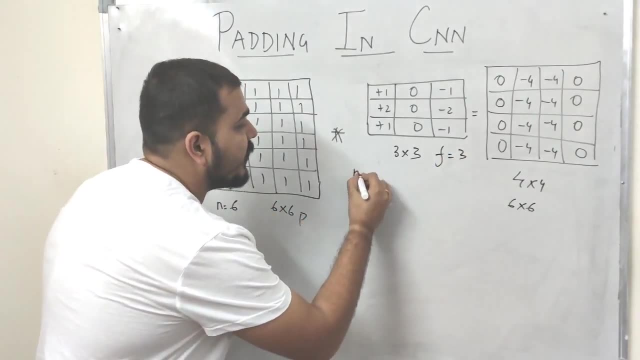 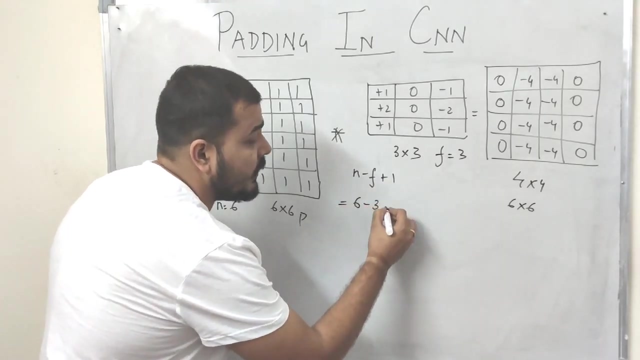 to the n value. so suppose my n? i'm saying that it is basically six, fix six pixels. here i'm basically saying that my filter size is three. so i showed you that one formula that i basically applies: n minus f plus one. here my n value is six, filter size is five. sorry, three plus one. 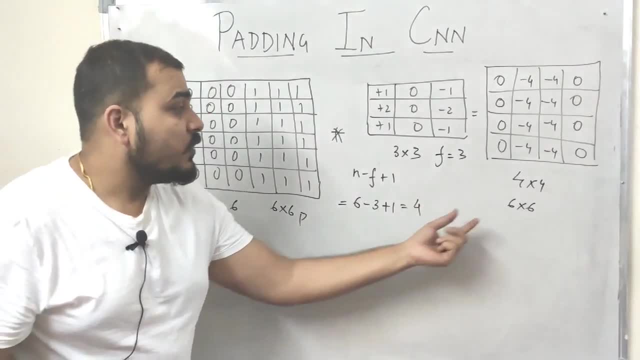 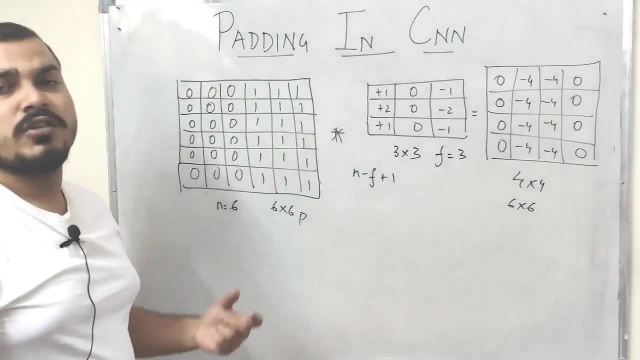 when i'm calculating this, i'm getting an output as four, and that is what this output dimension i'm getting. now what if i want to get the output dimension of six from my six cross six pixel? so here my output will be six. i have to calculate this n value. okay, now suppose, if i calculate the 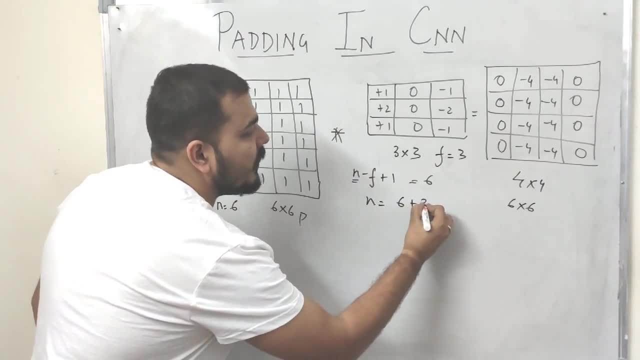 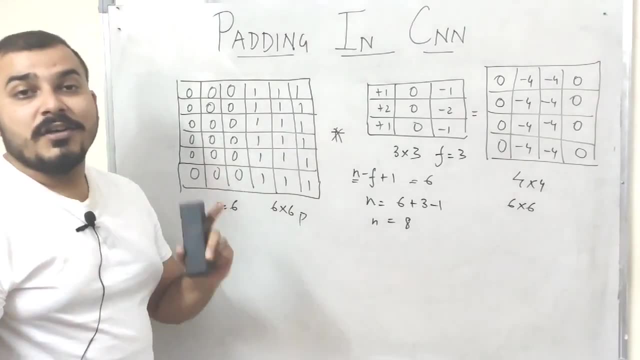 n value. it will be basically this: f will go over here and it will become plus three minus one and if i calculate, this n value will be eight. but you notice that we have six cross six pixel. how can we make it as eight cross eight pixels? that we need to think, and for that we'll use a technique called. 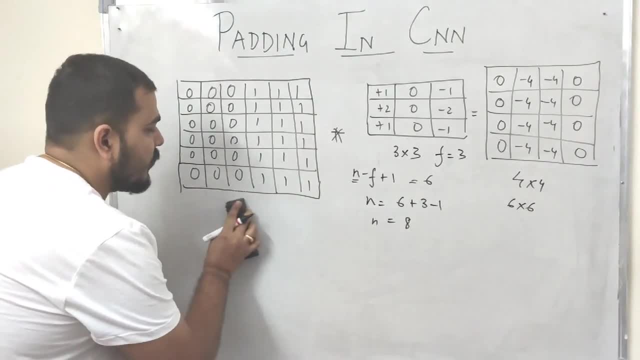 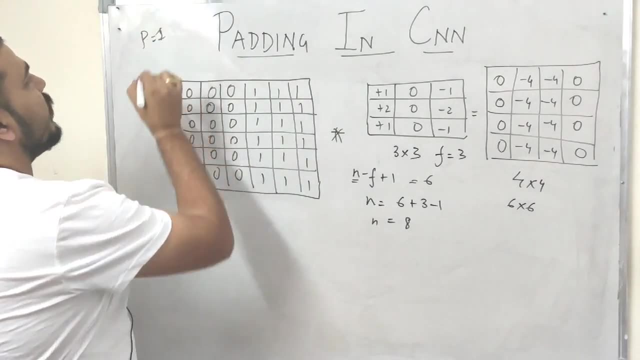 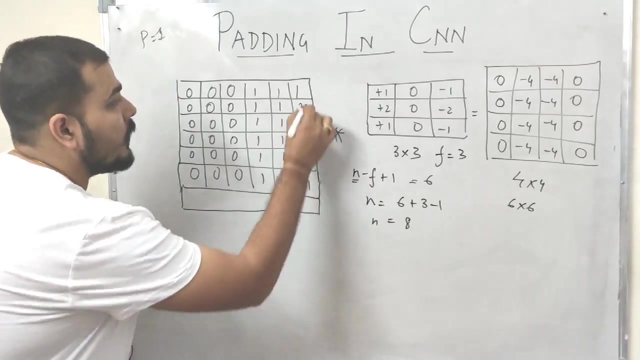 as padding. now padding what it does is that if i want to make this six cross six into, say, eight cross eight pixels, i'll add a padding of one. suppose i'm adding a padding of one, and what this does is that it tries to add one column. sorry, one row over here. another one column over here. one more row on the top. 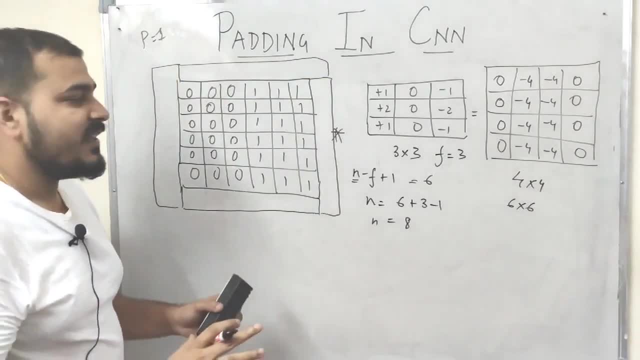 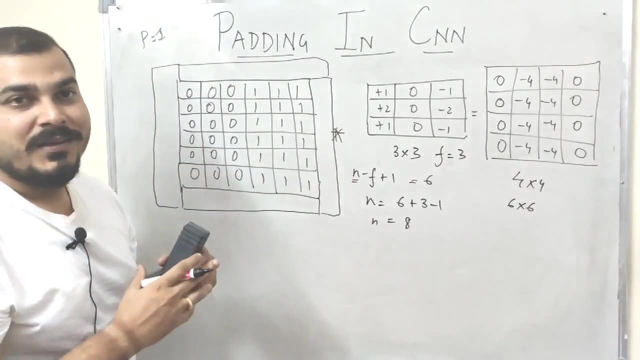 and finally, one column on the left. now, this is basically like you, you have your home over here, okay, and you are basically creating a compound on the on surrounding the home so that you don't lose anything from here, right? because you see that if i was just using six plus six, 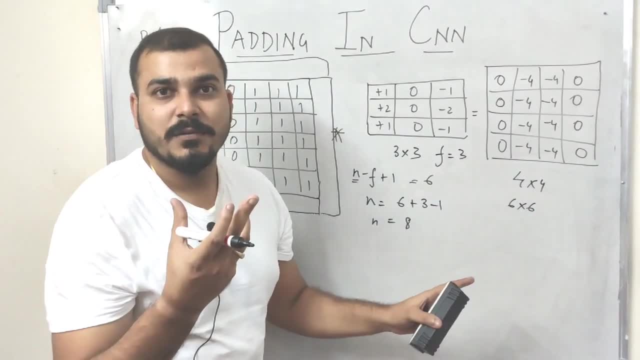 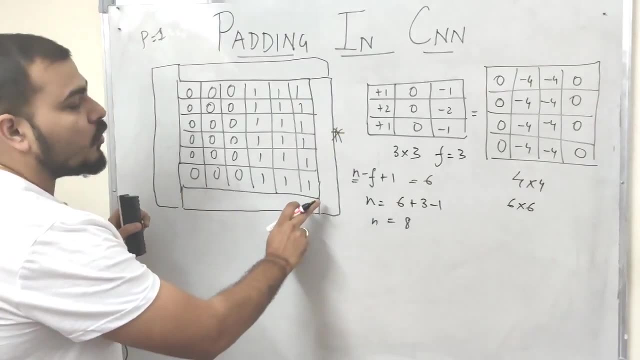 pixels. i'm basically getting four cross four output, so i'm basically losing some information. now what i have done is that i have just taken padding is equal to one, and i have basically created. i've added one row on the bottom, one row on the top. uh, one row, one column on the right hand. 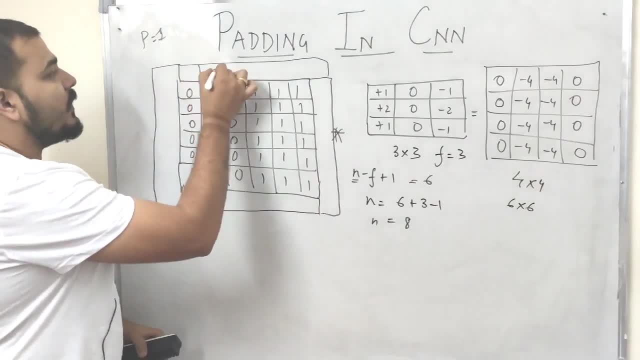 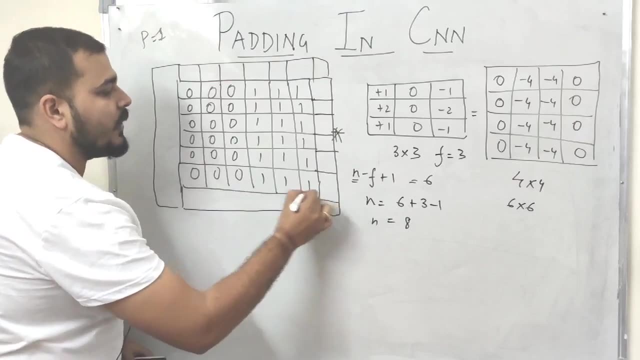 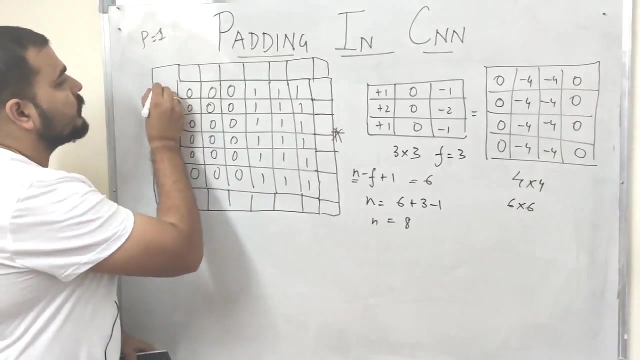 side and one row on the left hand side. now, this particular row will then- i'll just uh, join all these lines. it will now become eight cro eight cross eight pixels. this image will now become eight cross eight pixels. you see this? eight cross eight pixels. fine, now, when i have this eight cross eight pixels. 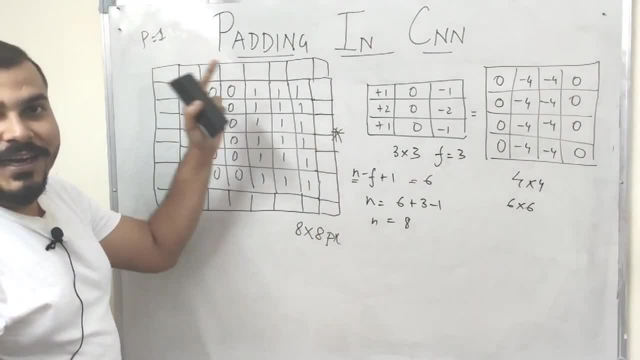 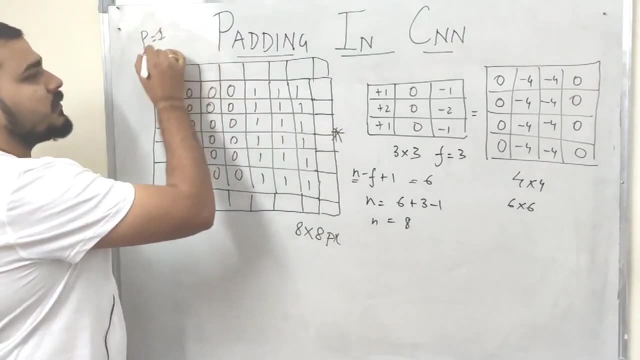 right, you can see that i'm having eight rows and eight columns now. now what value i can fill in? this is basically of two types. one is that you use g zero padding. you have something called as zero padding, wherein the first technique is basically called as zero. 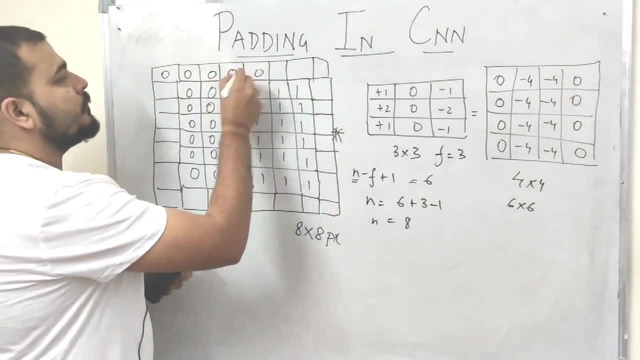 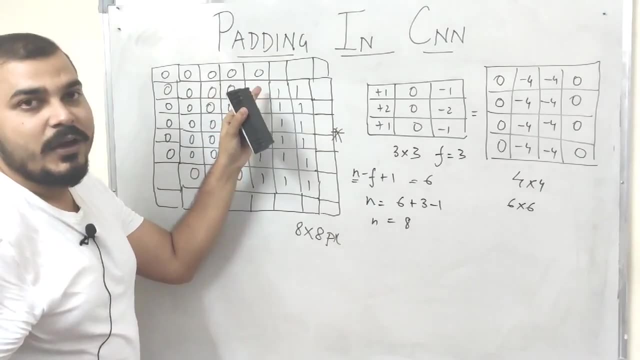 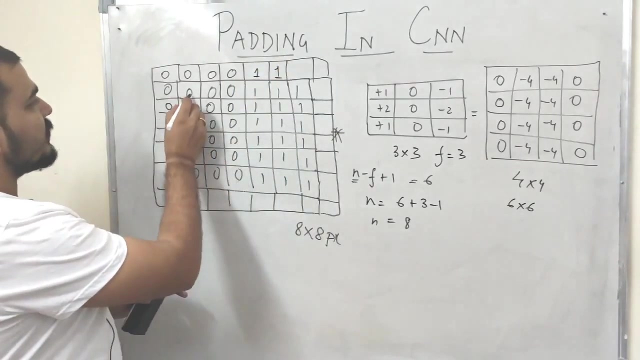 padding where you will just insert zeros everywhere, like this. the other technique is that you try to find out which is the nearest value and you try to put the same value. suppose this is your neighbor. right, one is your neighbor. you'll try to put one. one again one. suppose zero is your neighbor, you. 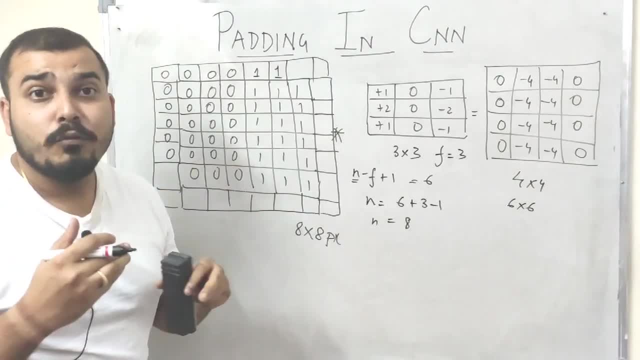 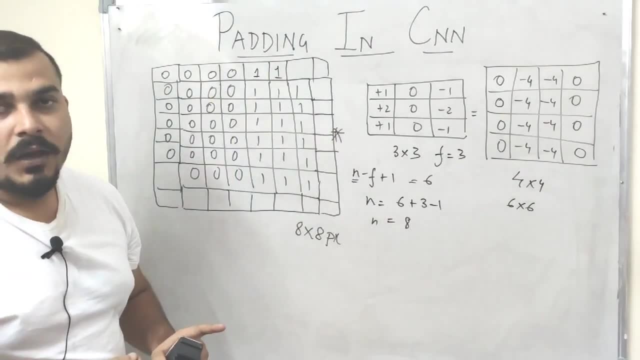 try to put zero. so most uh, useful technique, most commonly used practice, is basically that you'll try to use zero padding. okay, everywhere you will try to fill it with zero. okay, now, when you are using eight, cross eight, and now when you apply a filter is equal to three. you are basically going. 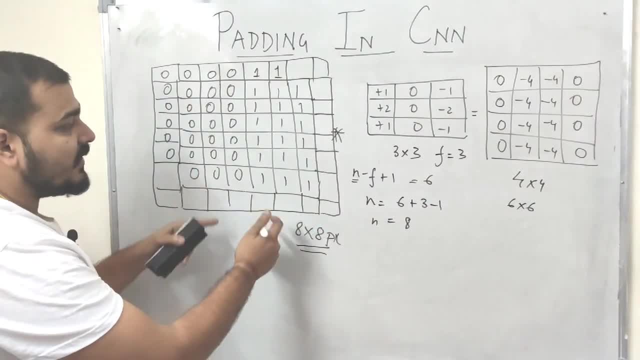 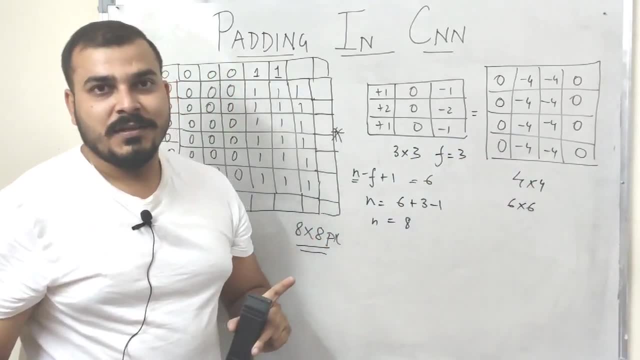 to get six cross six. right, because now you are going to get six cross six. right, because now you your image. just imagine that it was six plus six. you have added a padding on top of that, then you have applied a filter and finally your image output is six plus six. so now let us see that. 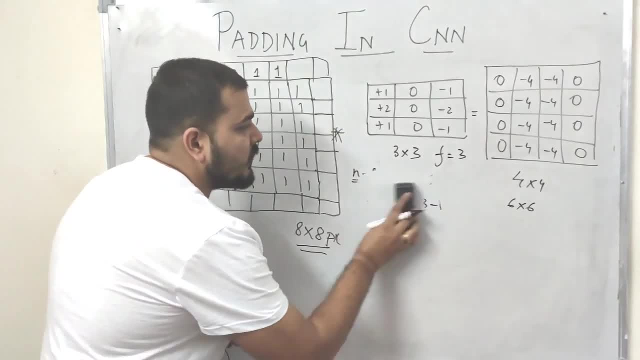 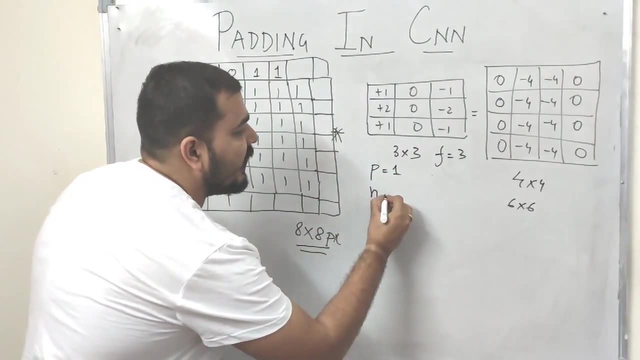 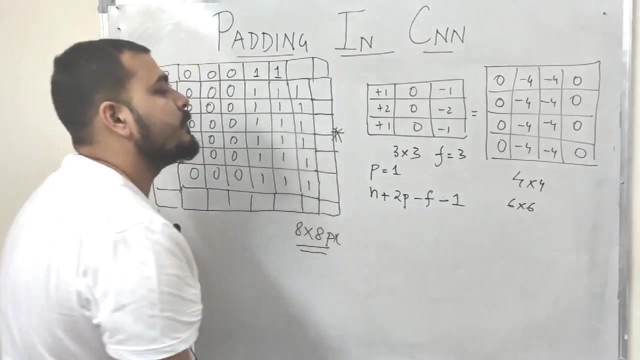 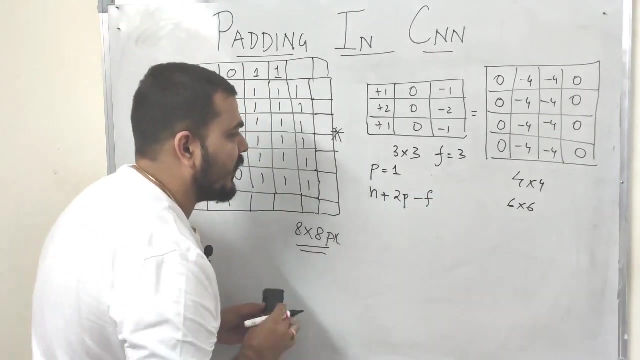 how this formula changes if i apply padding. so suppose if i'm adding a padding, value of p is equal to one. okay, so now my formula basically changes as n plus 2p minus f minus 1, n plus 2p plus 1. sorry, it should be plus 1 or minus 1, let me just think about it. okay, so n plus 2p. so let's. 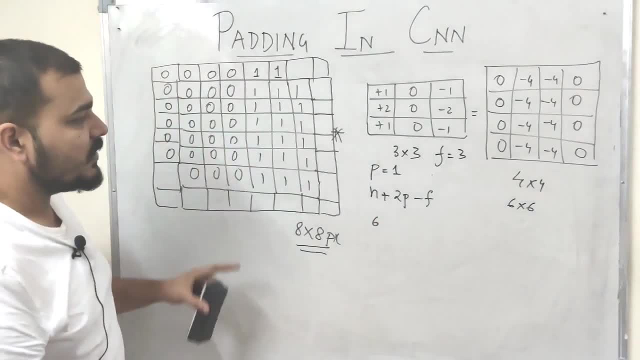 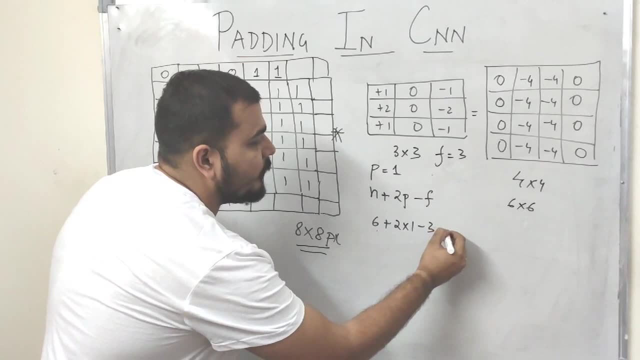 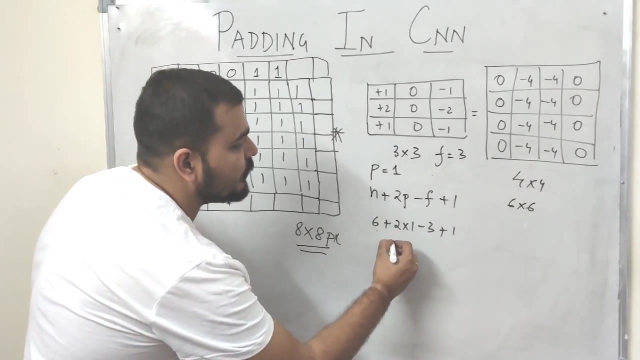 let's- uh, you know, n value is basically 6, because that was my original size- plus 2 multiplied by 1 minus 3. right now, when i am multiplying this, it becomes 8. okay, it should be plus 1, sorry. so when i'm multiplying 2 cross 2 multiplied by 1 plus 6, it is basically 8 minus 3, which is my 5 plus 1. 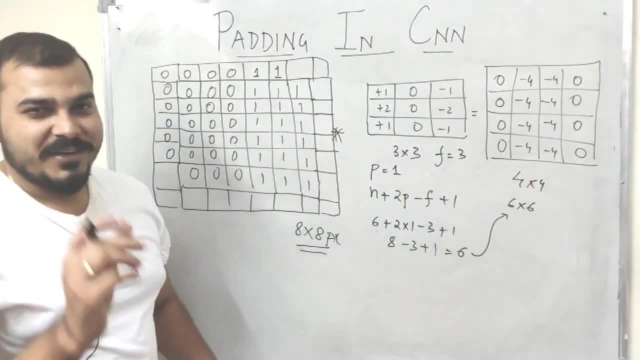 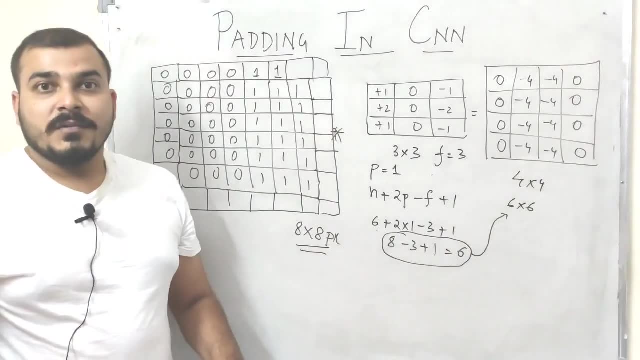 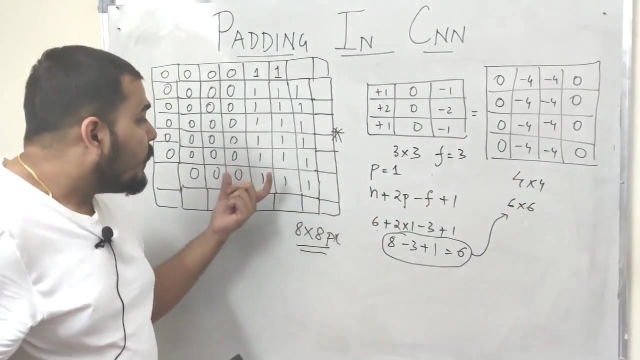 which is equal to 6.. okay, i'm sorry because of this little bit confusion, so i've just made it as plus 1. okay, so when i apply this particular operation now, i'm able to get six cross right now, understand guys here, based on the type of output. right, if you try to apply this particular formula, you will. 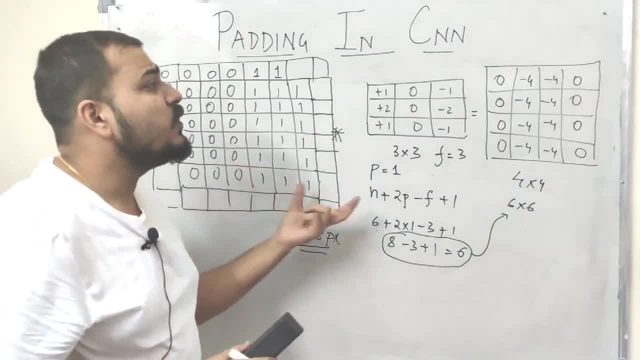 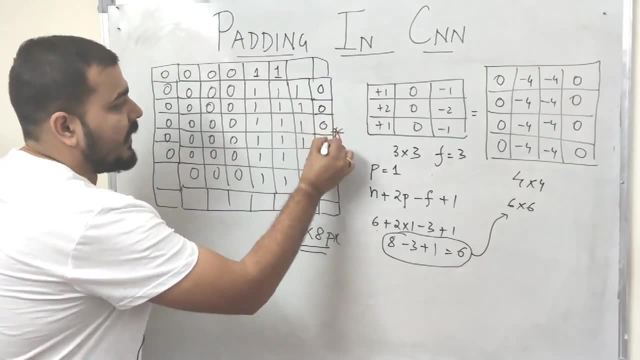 be able to get the same pixel of the image size, so that basically means you're not losing much information. in addition, you'll be able to get more edges. how see when, i suppose, if i'm using zero padding over here and when i apply this filter, this is one more edge right. 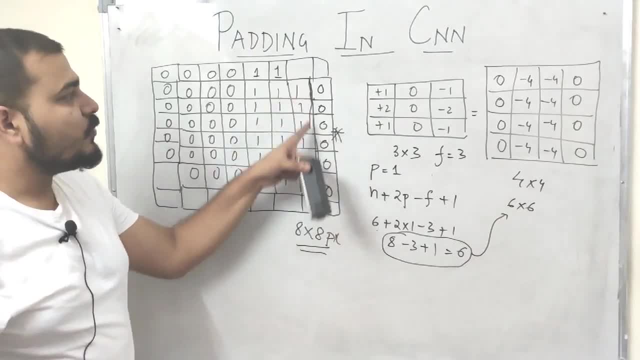 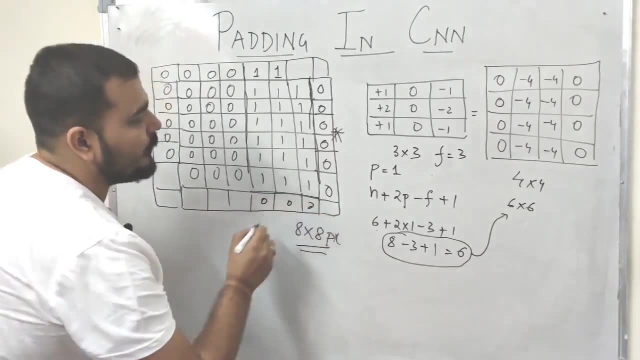 you can see that this ones are here, zeros are there, so this becomes one more edge. and this, this is also one more edge. right, this is also one more edge. and suppose, here you also you're putting zeros, this will also become one more, uh, horizontal edge. but currently i'm just basically seeing. 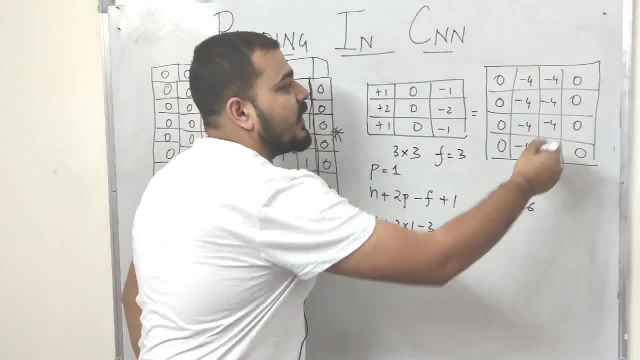 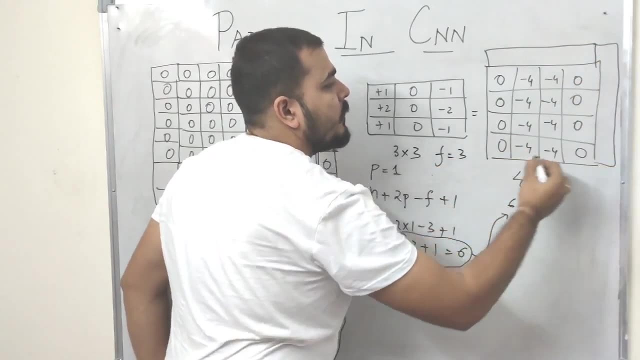 which will be the vertical edge. so i'll be able to find two vertical edges in this and i'll be able to get six cross six, okay, and again here. also, one additional row will get added. everywhere, row and column will get added and your output will look something like this: 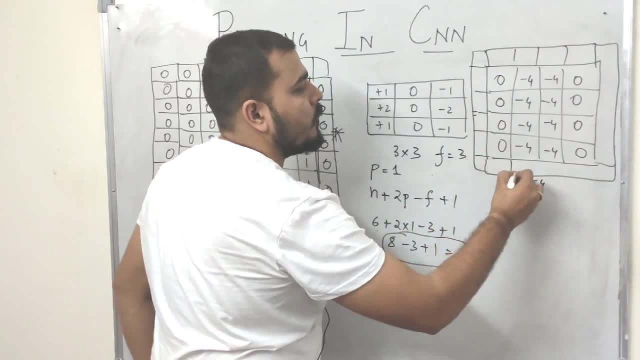 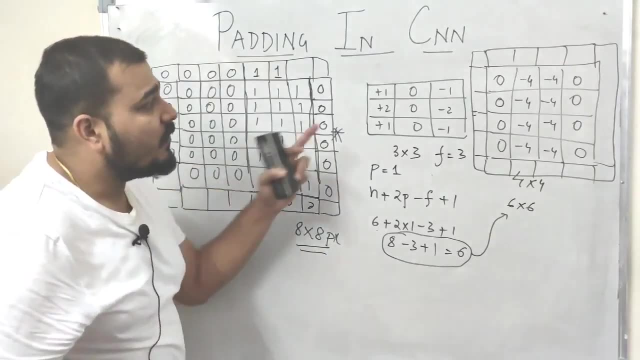 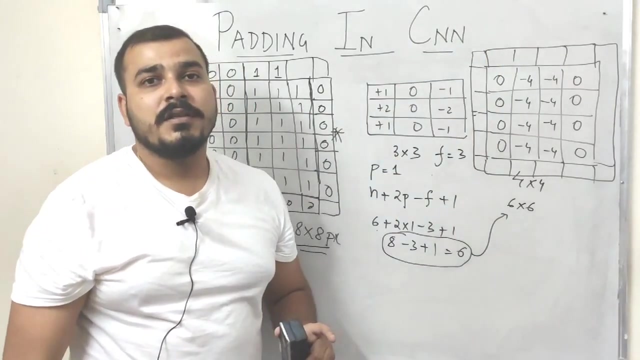 will be six cross six. so you should try to use padding, because it will actually give you the same image size after you apply a filter operation. that basically means now you can continue creating number of many, number of convolutions based on your image size, based on the types of filters that you want to.